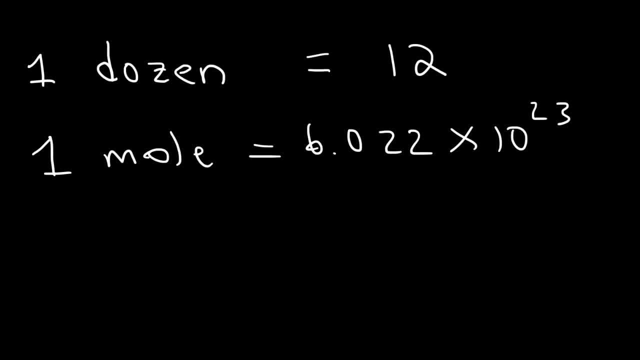 So you could represent a large quantity with a very simple expression, And so that's the basic idea behind a mole. It's simply to represent a large quantity of something, Which is very useful in chemistry when you're dealing with atoms, molecules and particles. 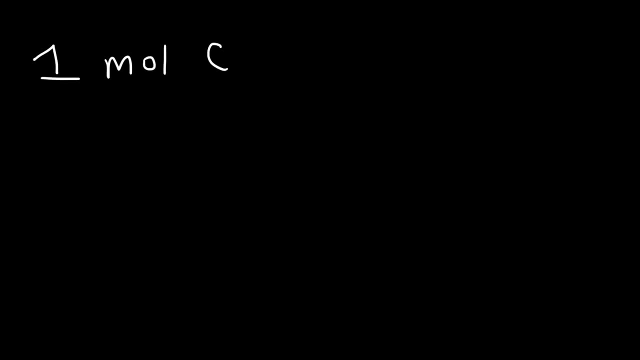 So let's say, if I have a mole of carbon atoms, What that means is that I have 6. Times 10 to the 23 atoms of carbon, So I have a large number of carbon atoms. If I have 2 moles of carbon atoms, then I have 2 times. 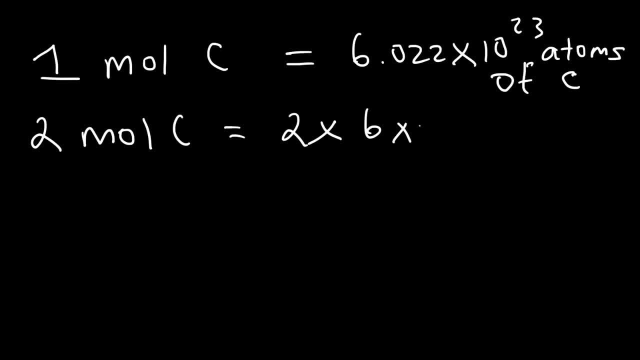 I'm going to round this to 6.. I have 2 times 6 times 10 to the 23 atoms of carbon. Let's say, if I have a mole of carbon dioxide, CO2 is a molecule. So what this means. 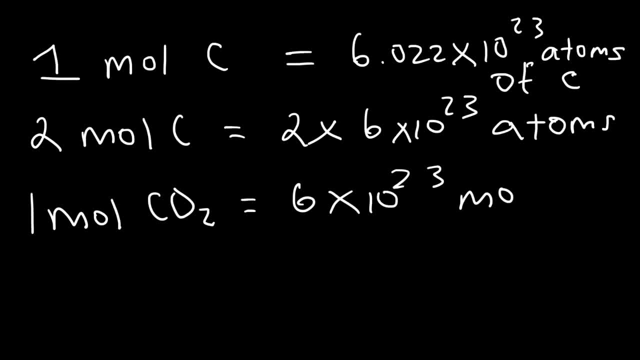 What this means is that I have 6 times 10 to the 23 molecules of CO2.. So a mole, as you can see it, represents a large quantity of particles, Or anything else for that matter. Now, sometimes you may need to relate moles to grams. 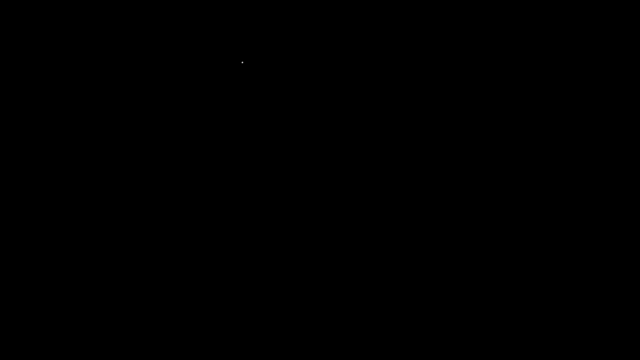 You can also relate moles to grams. Consider the element nitrogen. On a periodic table, nitrogen has an atomic number of 7 and a mass number of 14.. We're going to focus on the mass number, Which you can also represent as 14 atomic mass units. 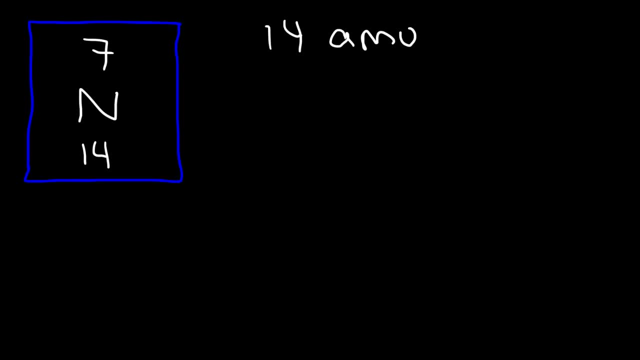 The number 14 also represents something called the molar mass. It's 14 grams per mole. Now think about what that means. 14 grams per mole, So that means that 1 mole of nitrogen has a mass of 14 grams. 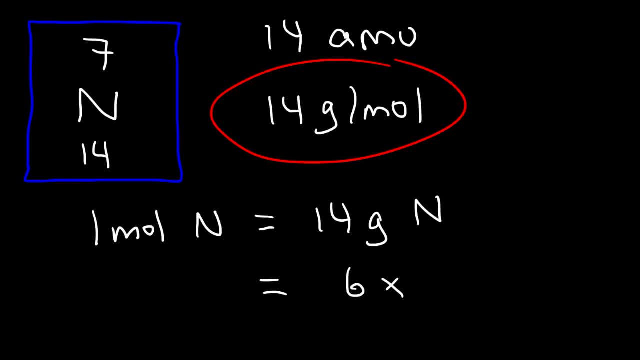 And we know that a mole is 6 times 10 to the 23 atoms Or particles or molecules. But n is just an atom. So 14 grams of nitrogen contains 6 times 10 to the 23 atoms. So now you can connect everything together.